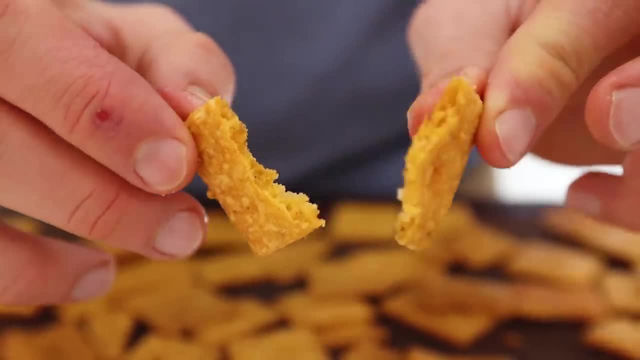 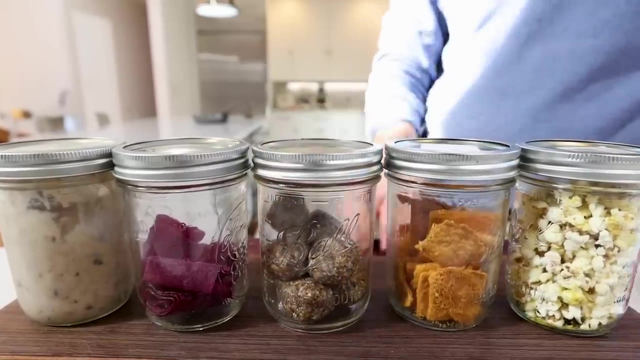 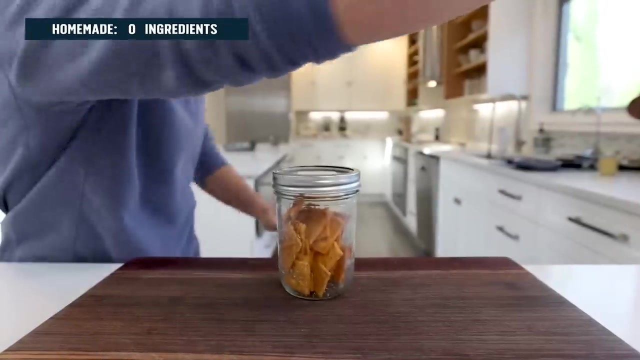 to satisfy your sweet and salty craving, but they're going to do it in a much more sustainable way, because they're all completely made from scratch and they all come together with just five ingredients each. All right, first up are these cheese crackers. Now these have become. 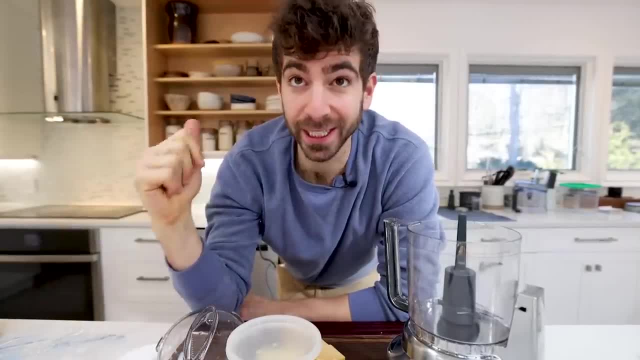 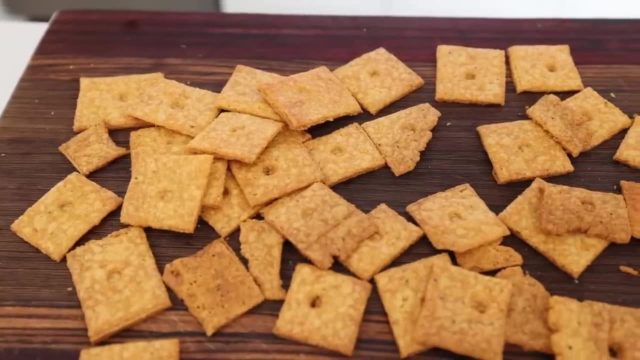 my absolute favorite in the last Oh Oven preheated. First step: preheat your oven to 350 degrees. Thank you, beeper. These have become my absolute favorite in the last three, four months. I've been making them Every other. 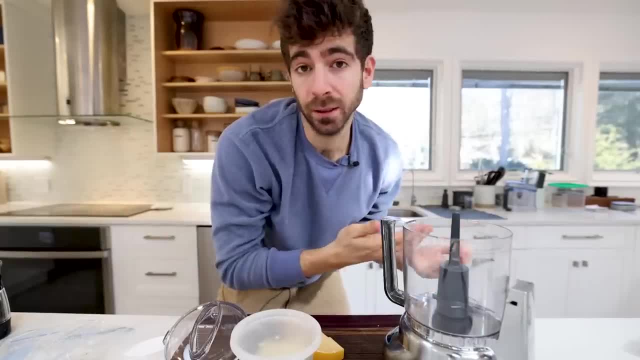 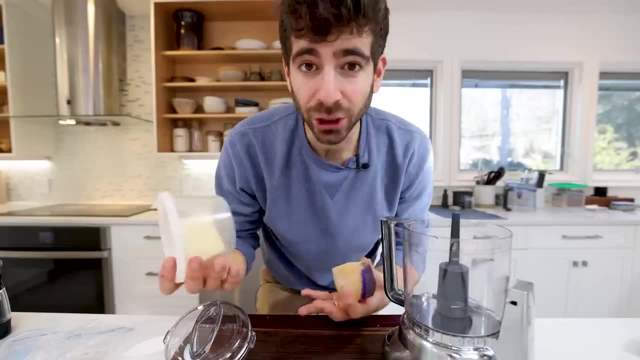 week. I would say You would think making crackers from scratch would be a little difficult, but it's really not. It's actually really simple with this method. Now it all starts with cheese- Really any cheese you want that's going to have a nice melting consistency. Cheddar, classic, obviously. 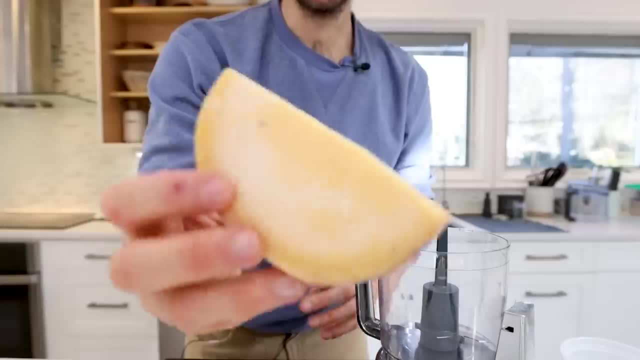 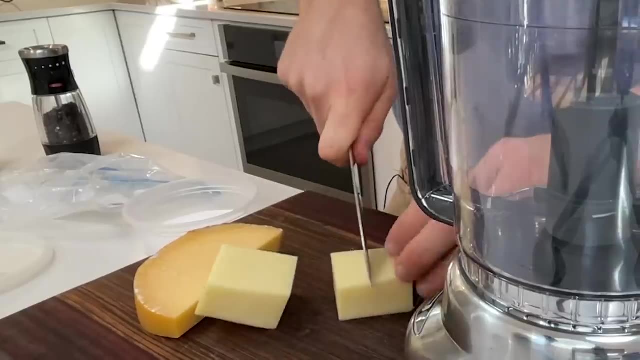 If you want them to be yellow, use a yellow cheese. This, I don't even know what. I don't know what this is. My mom brought this up and left it here, but I like it. It smells good. It's going in these crackers. Cut this into chunks so it processes easier. 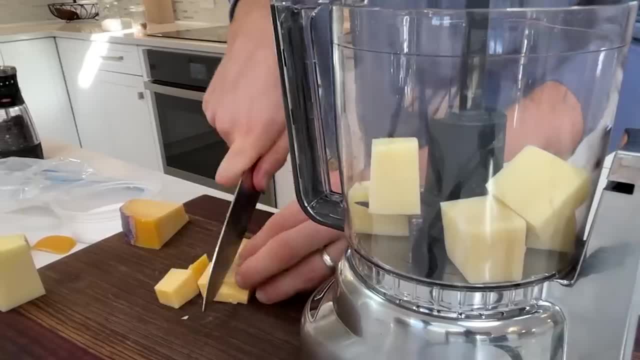 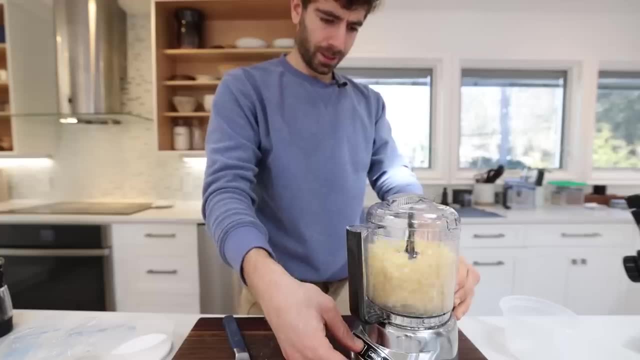 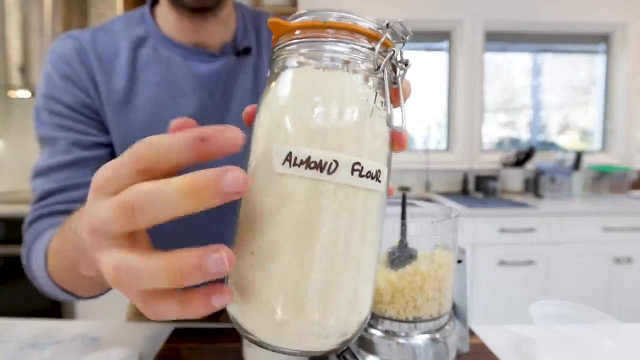 So, like all of these snack recipes today, I just eyeball the amounts, but if you want exact ratios, just click the blog link below. Now we process. You just want it crumbly like that. Now for your flours, you really can use anything. I'm going to make these gluten-free. 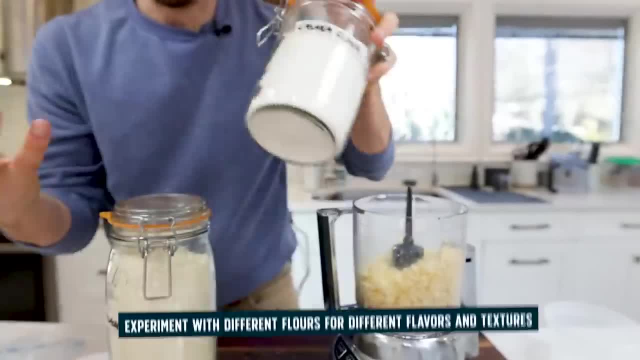 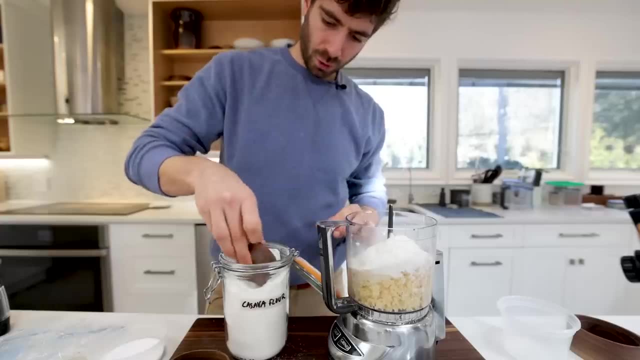 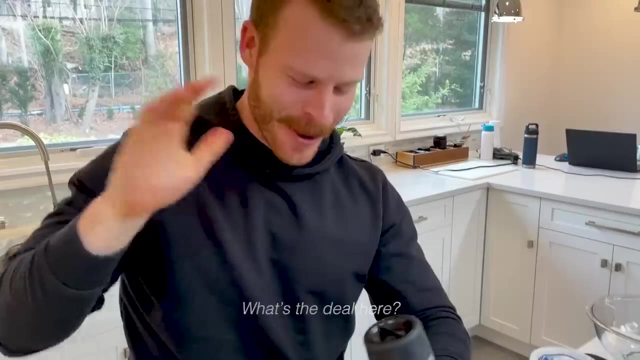 with some almond flour and a little bit of cassava flour- But feel free to use actual wheat flour- Going in with about a half cup of almond flour, about a quarter cup of cassava flour. Finally, a whole bunch of cracked pepper, Ethan style, The cracked pepper king. A little bit of spice. 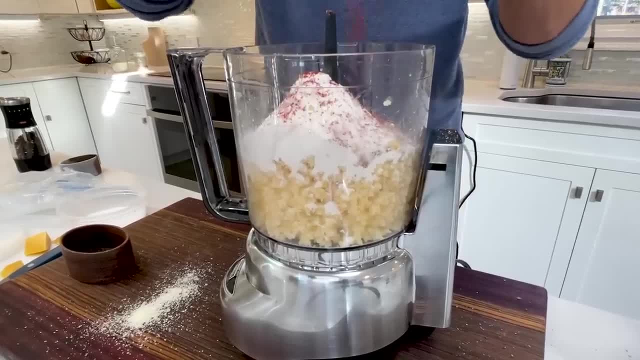 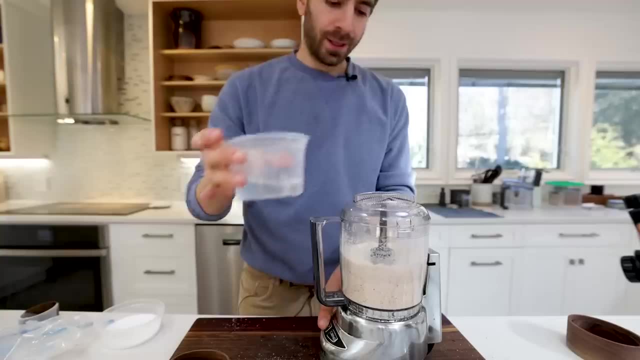 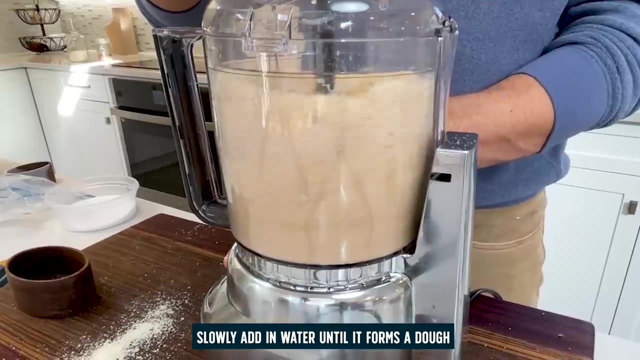 Paprika. You can use herbs in this Rosemary thyme. That's going to be great, Totally customizable. And then, finally, some salt. We'll get some water, We'll start blending and then slowly strain, And then we're going to cream in your water. Check, it Actually smells great There you. 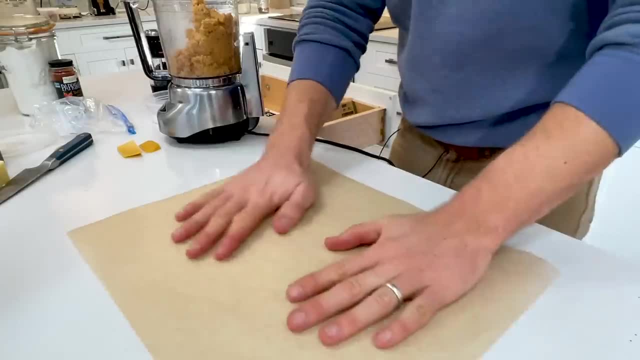 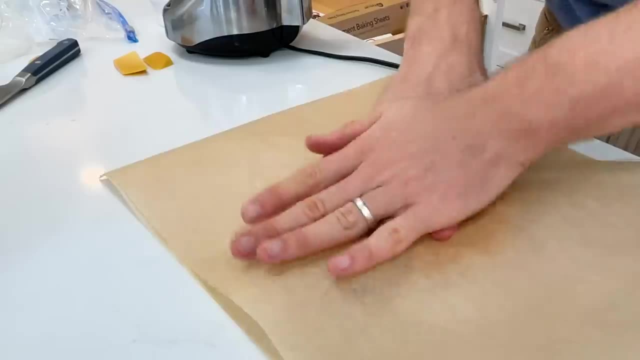 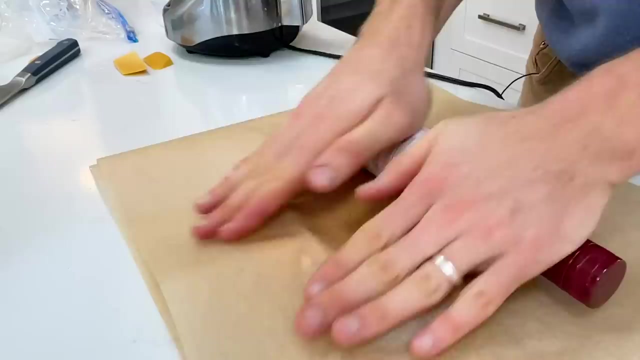 go. That's a nice dough right there. Now watch how easy it is to roll these out: Parchment paper Plop. Just form that into a ball. Another piece of parchment paper or plastic wrap. Don't think I have a rolling pin. I don't have a rolling pin, so this will do. Oh it's. 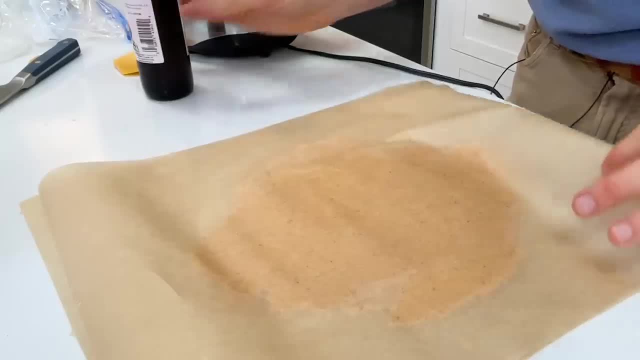 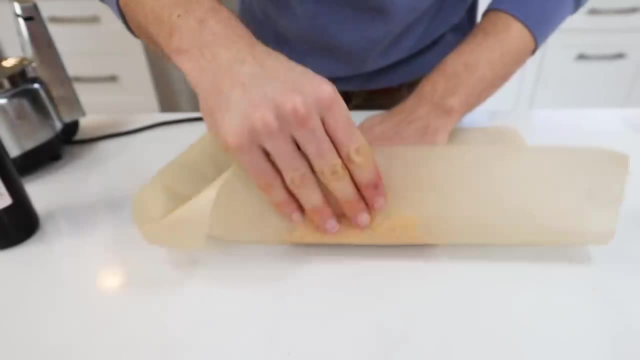 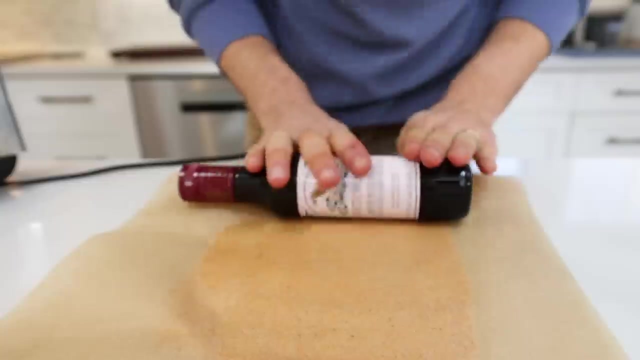 not the best. So just start rolling it, And when you get about here, See how rough those edges are. Fold and fold and fold and fold A little square. Now back on, Roll into an even rectangle. I don't know what the exact measurement is, Maybe between 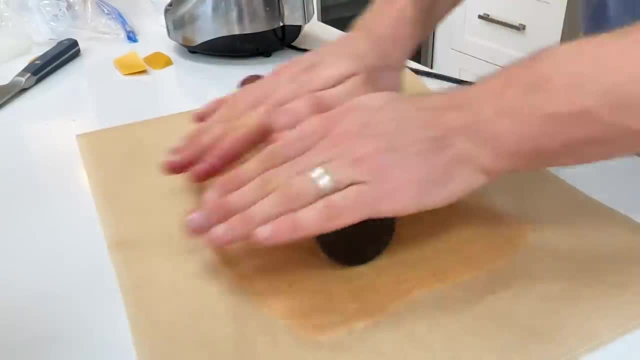 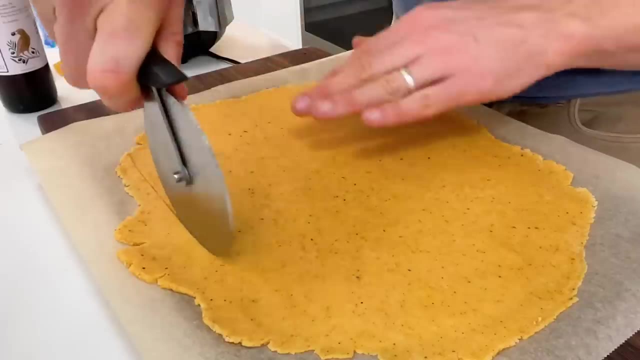 an eighth and a quarter of an inch. No one wants a thick ass cracker. You want a nice thin, crispy cracker. Take a peek, I'm happy with that. Slide this onto a cutting board And some crackers, That's it. 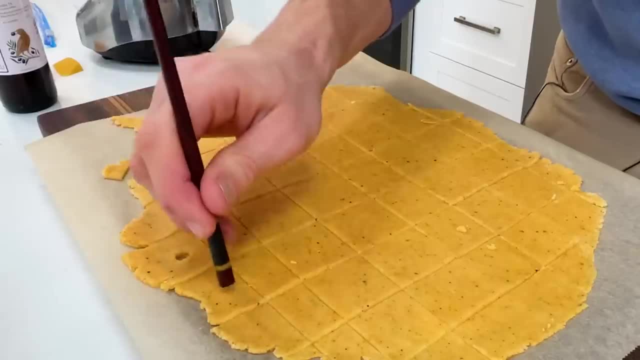 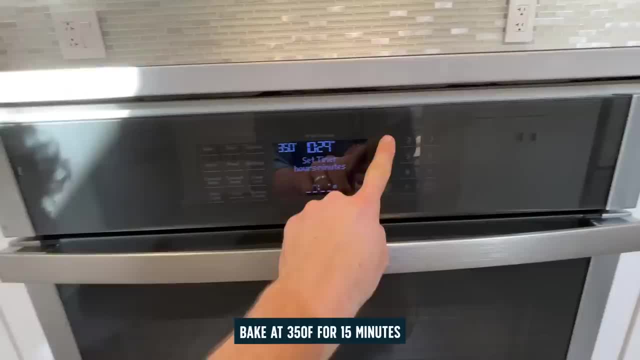 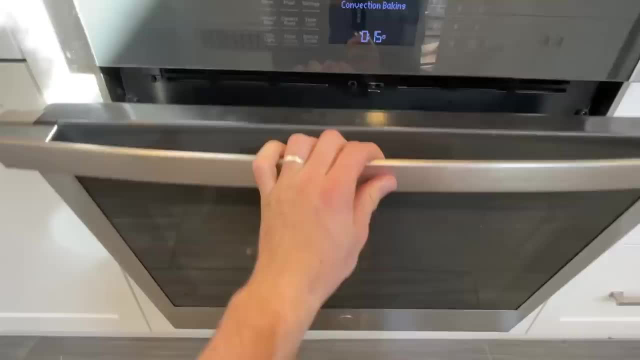 sheet. Like I said, oven preheated. Throw that in there. I'll bake for fifteen minutes. Now, once these have cooked a bit, they'll be able to break apart, and then I'll cook them again to get those edges crispy. 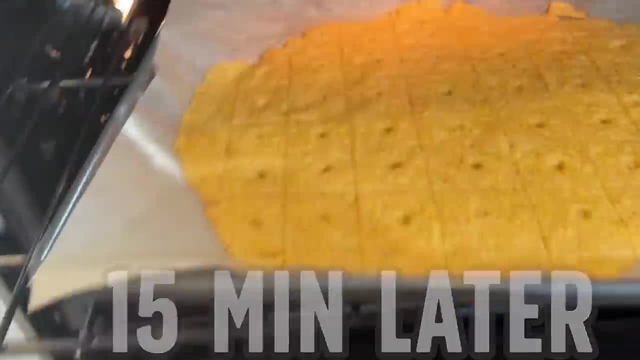 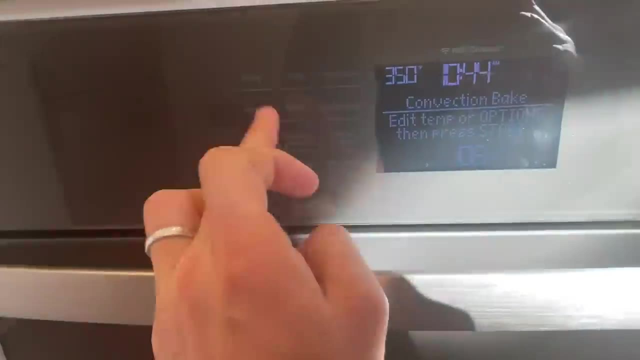 Right, 15 minutes up Looking at these: Wow, They've got some bubbles. They puffed up just a little bit Looking good, So I'll pop these here, Turn the oven up just a bit to 30 degrees And we're ready to use them. 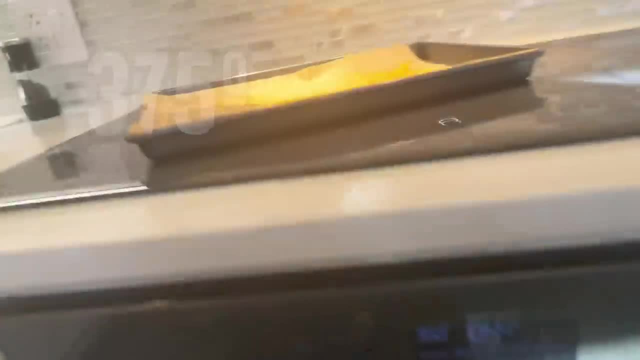 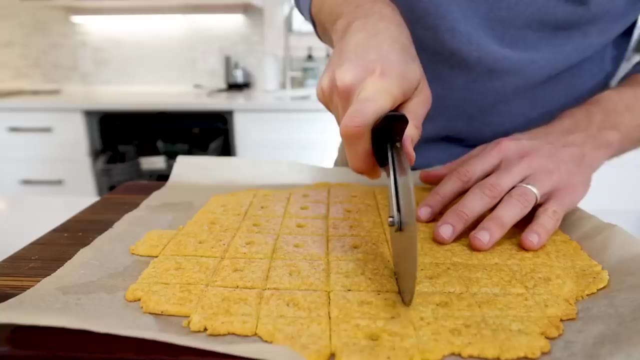 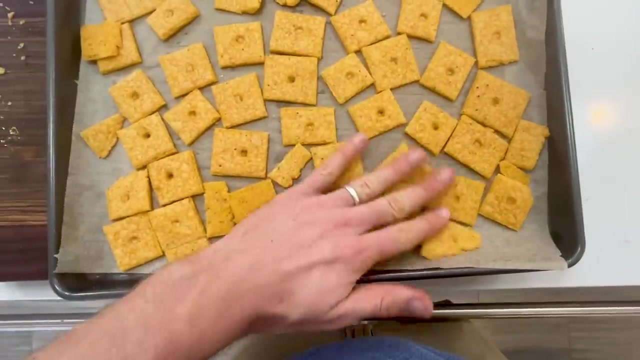 three, seven, five Fahrenheit, And I'm just gonna retrace the lines, pushing a little harder this time, This way Back on. Oh, now you can see those break right apart. So the goal here is just to give each cracker. 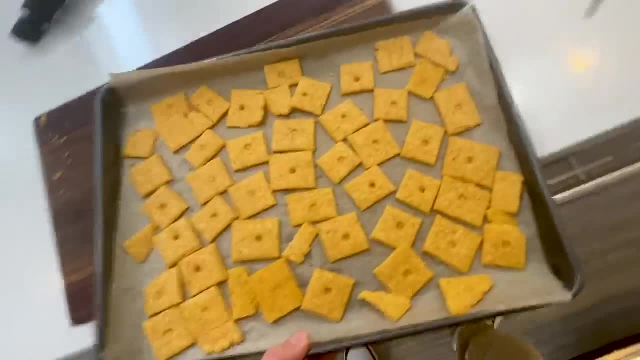 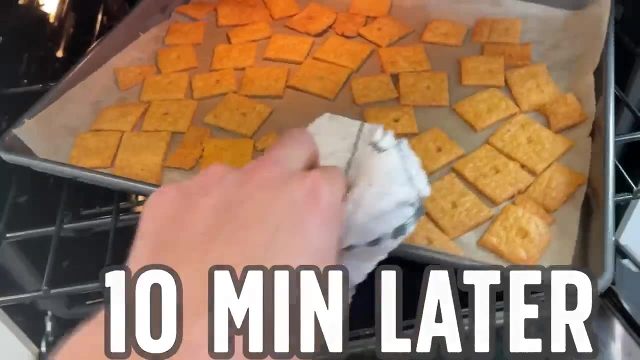 a little bit of room between the edges so they get that crispy side And back in the oven. I would say those only need like five minutes, All right, so these actually took 10 minutes to cook in here. Let's see on the undercarriage. 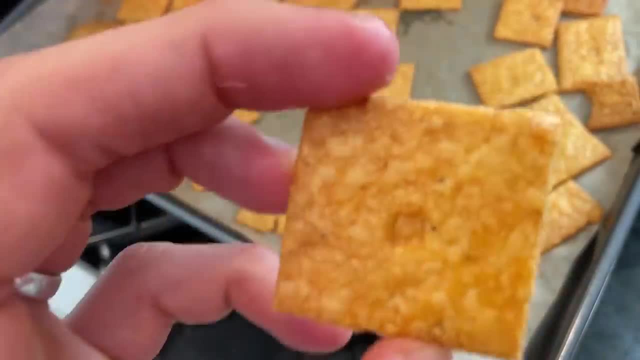 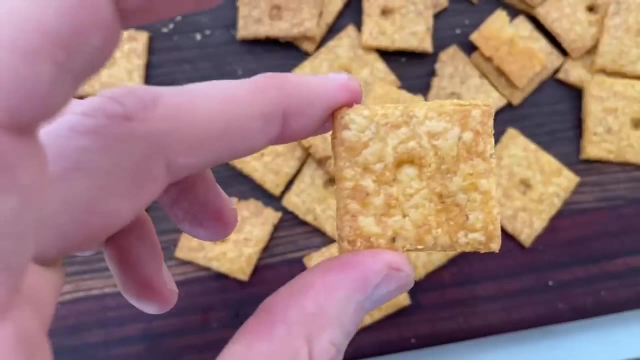 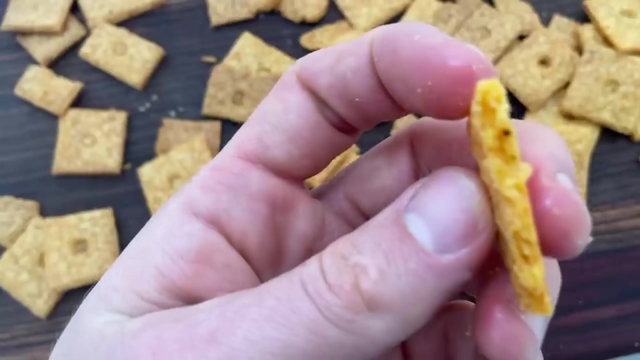 Now that's crispy. Wow, Bubbly, just like a Cheez-It. Now the nice thing about hand rolling is that some will be a little bit on the chewier side, the thicker ones, and then some like this: That's super crispy. 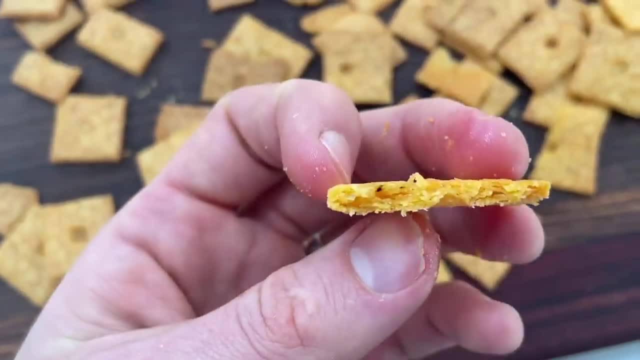 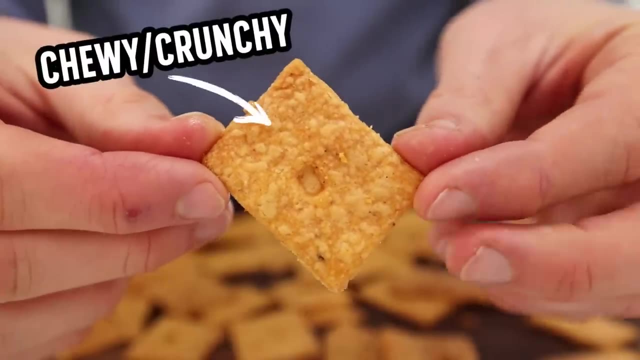 But it's amazing that you get some flakiness in there. Actual taste test: Mm. Okay, that one was the perfect texture blend between chewy and crunchy. It's amazing that you can make a cheese cracker like this with just a few ingredients. 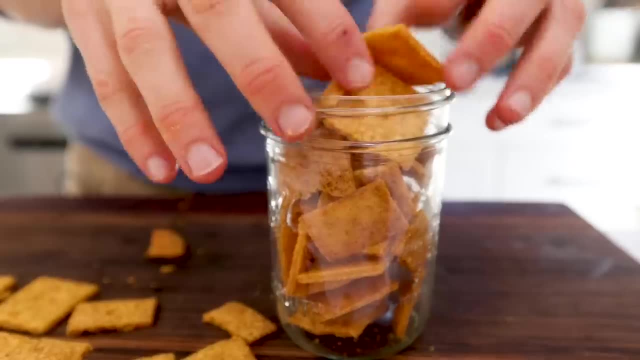 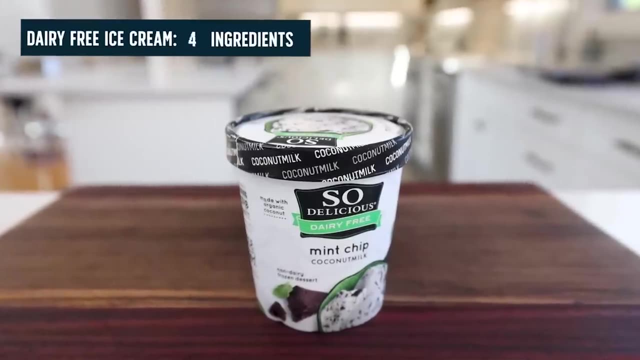 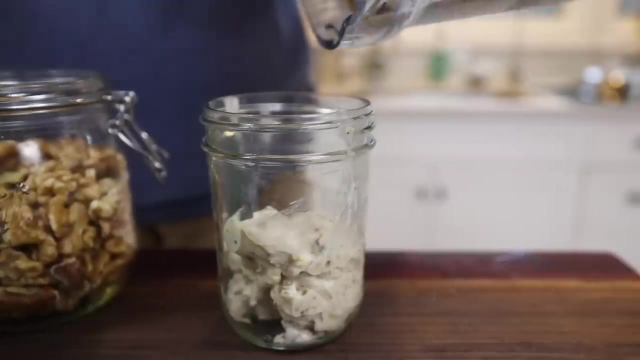 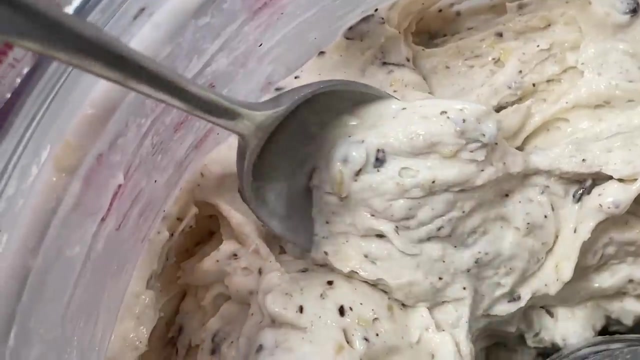 These are salty, they're satisfying and they're great to have around in the pantry. So you can't really call this ice cream per se, but this is by far my favorite frozen dessert because one it's incredible. but more importantly, 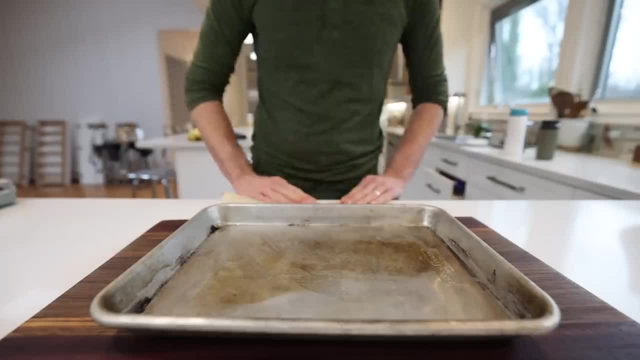 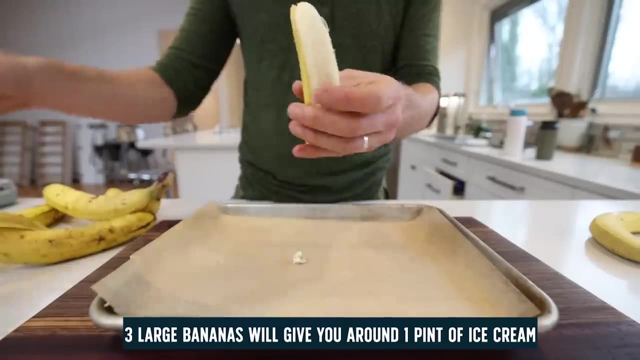 you don't need an ice cream maker. First thing I'm gonna do is freeze some bananas. Generally, three larger bananas will give you a good pint of ice cream, which is how much I tend to make at one time. I'm gonna rip the bananas into pieces. 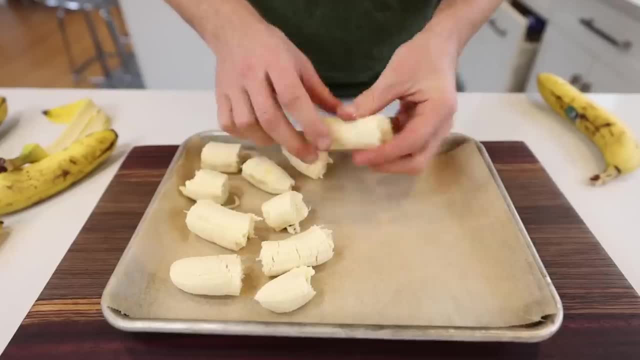 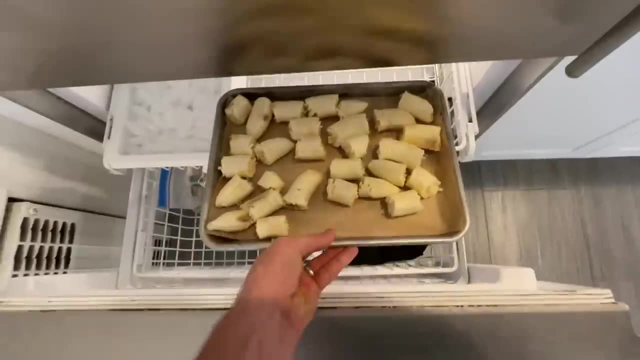 and pop them on a baking sheet with some parchment paper, making sure they're not touching to avoid clumping together when they actually freeze, And then I'll toss them in the freezer overnight. But if you're really pushing it, you could probably get away with freezing these. 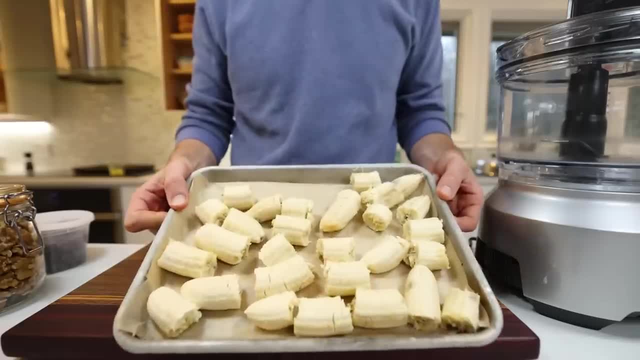 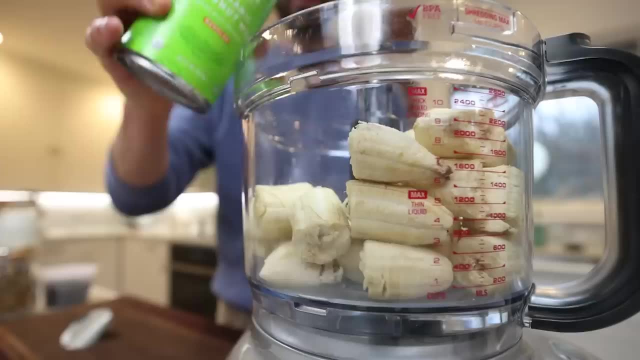 for four hours, at least That minimum. Once the bananas are frozen, I'm gonna add them to a food processor along with some coconut milk to add a little extra creaminess and up the fat content. But really you could use any milk or fake milk product. 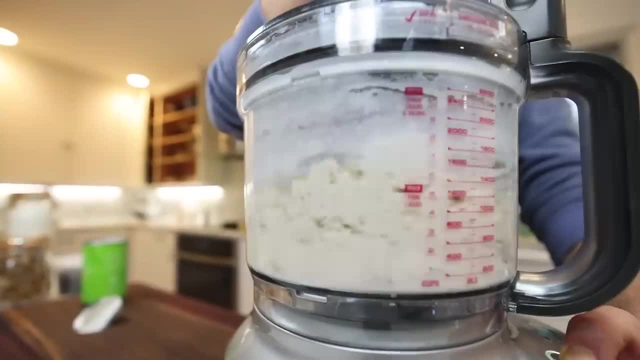 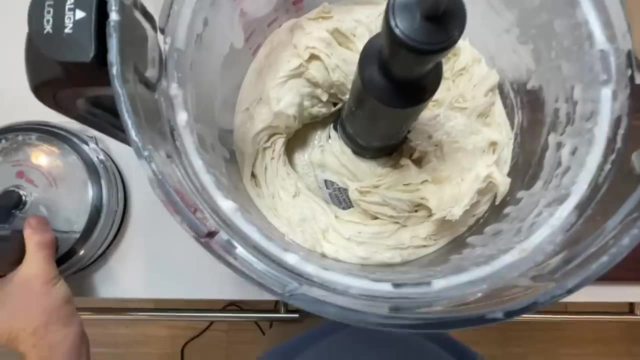 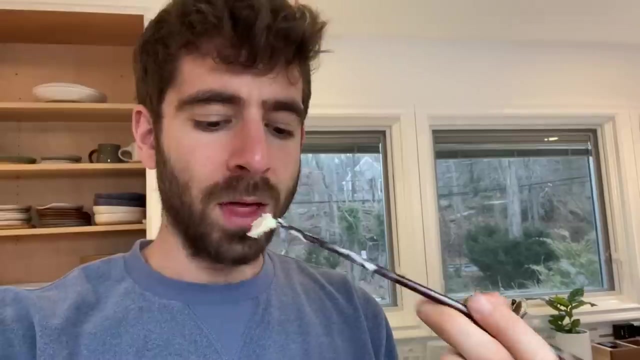 that you have in your pantry or you prefer, And then blend to creamy perfection. Let's take a peek. Wow, look at that ice cream consistency. That is silky right there And that looks like straight up gelato. Wow, Two ingredients. 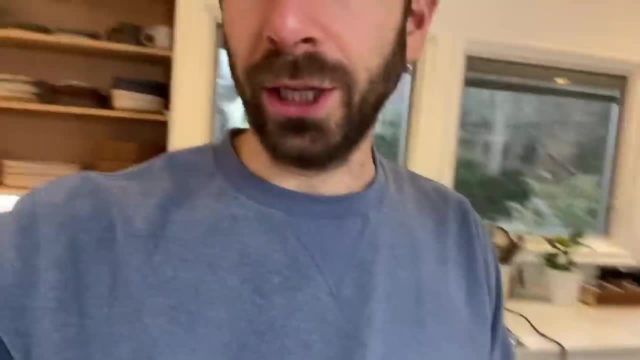 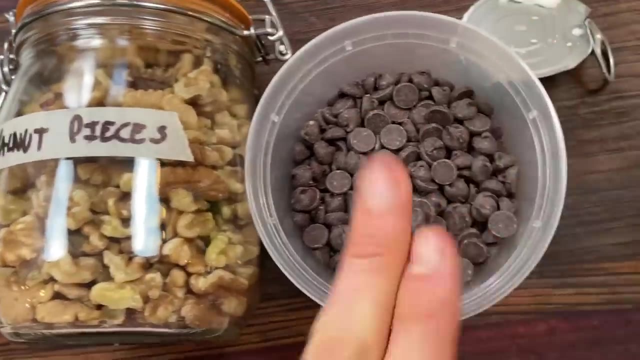 Never tasted so good. Now that is creamy and delicious. But there's two more things I wanna add. You top it with whatever you want. For me, I really like this combo: Walnuts- chocolate- These are actually Stevia sweetened chips. 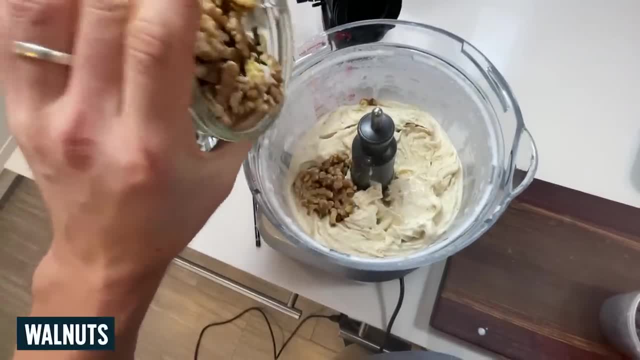 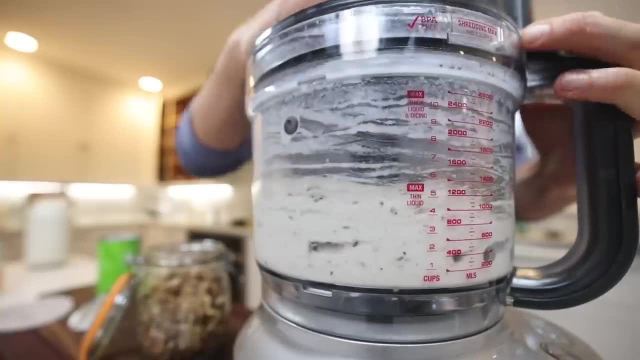 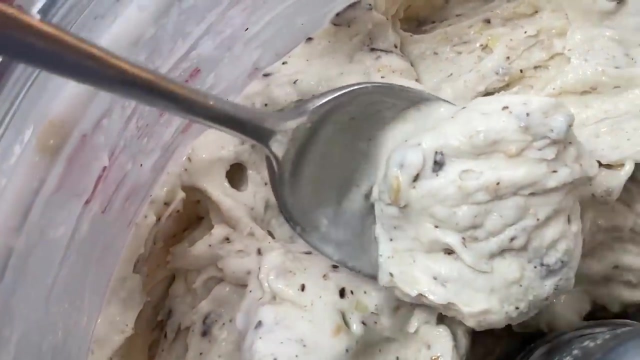 Make it just a little healthier, And what I'm gonna do is just add some walnuts chips And then I'll just give it a few pulses. Okay, now, it was good before that, right there: Bananas, coconut, walnut chocolate. 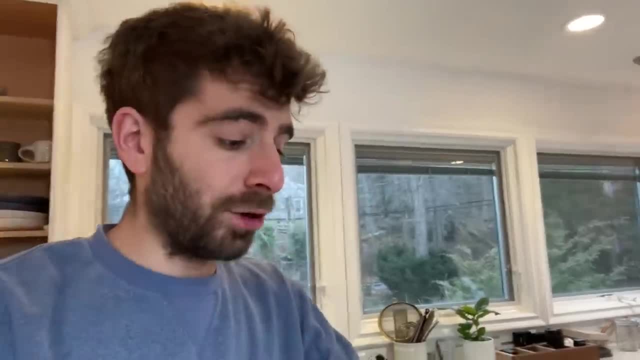 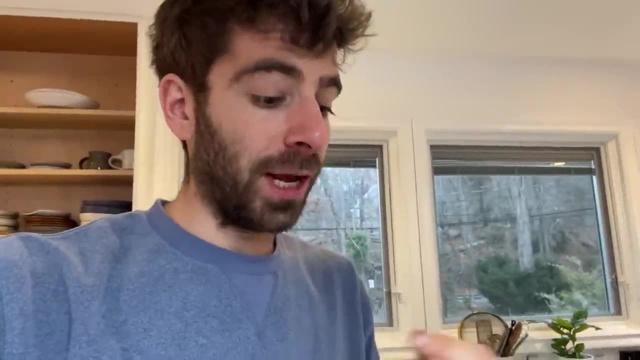 Four ingredients actually. So, honestly, when you have a fake ice cream like this, it's a long shot to compare that to a cream and sugar base like a real ice cream base. which is why adding some textural elements, adding some more flavor with the nuts and the chocolate, 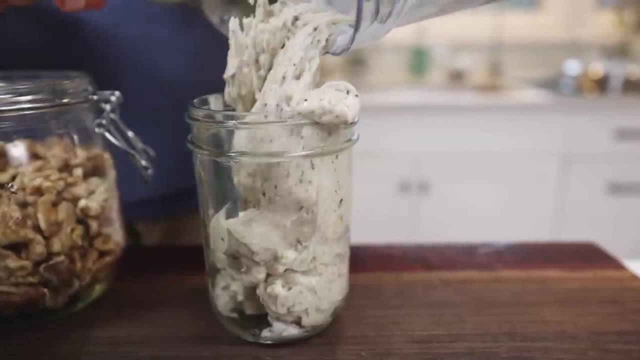 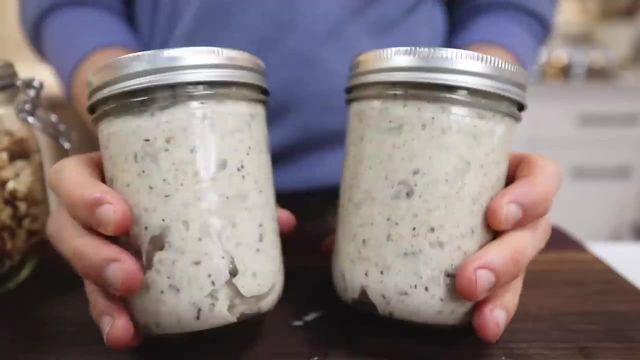 to me. it kind of needs that to really hold up. And this is holding up great. I'm not missing a dairy-based ice cream at all. So if you've been following the channel for a bit, you know I moved into this kitchen a few months ago. 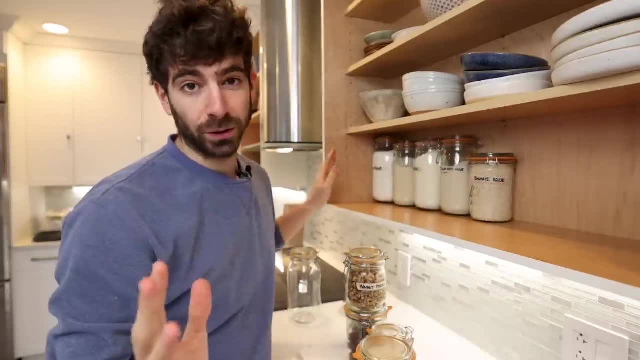 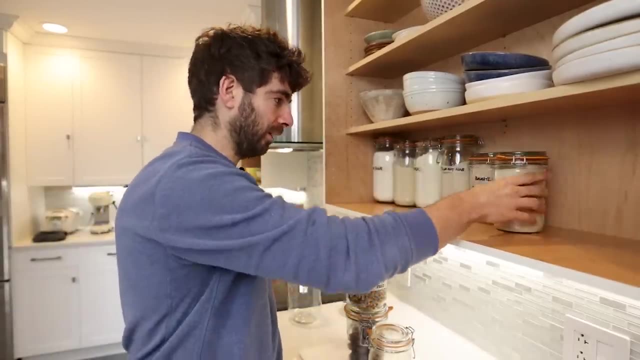 which is why you see these exposed cabinets. I just took the doors off. This is temporary. I'm actually doing a bigger renovation next month, but I couldn't live without some exposed shelves because I like being able to see my options, which brings me into the sponsor of today's video. 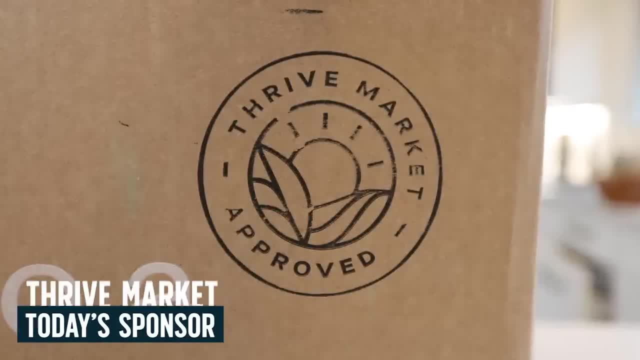 Thrive Market. Thrive is an online marketplace on a mission to make healthy living easy and affordable. Now, as a pro home cook, my goal is to create a culture, and I'm gonna show you how to do that. I'm gonna show you how to do that. 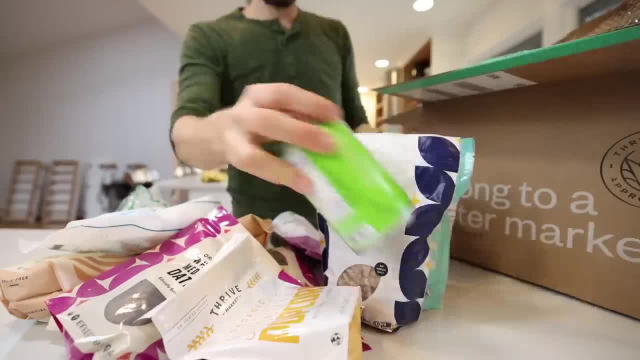 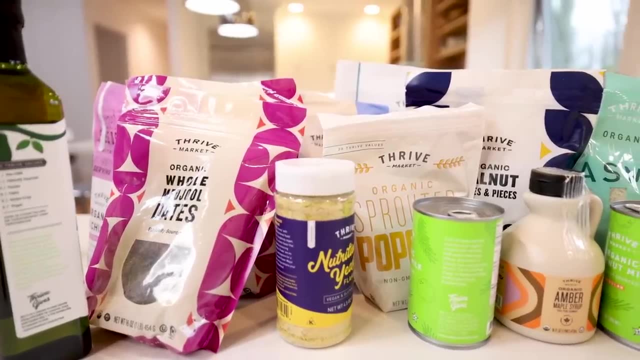 I'm gonna show you how to create a cooking environment that enables me to produce healthy meals- and in this case, snacks- on a daily basis. At Thrive, you can find everything you need, from those organic essential pantry goods to clean beauty supplies and even non-toxic cleaning supplies. 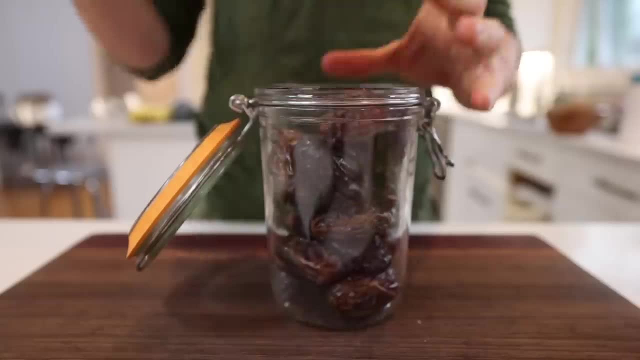 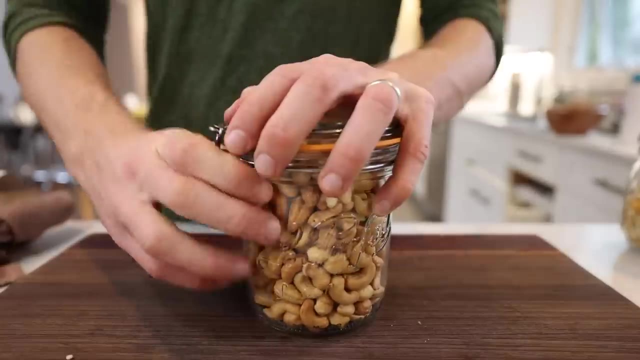 And the shopping experience is super streamlined, where you can filter out products by either your personal values or dietary preferences. But, most importantly, I trust that Thrive products are high quality, which puts me at a big headstart when I'm making all of these snacks completely from scratch. 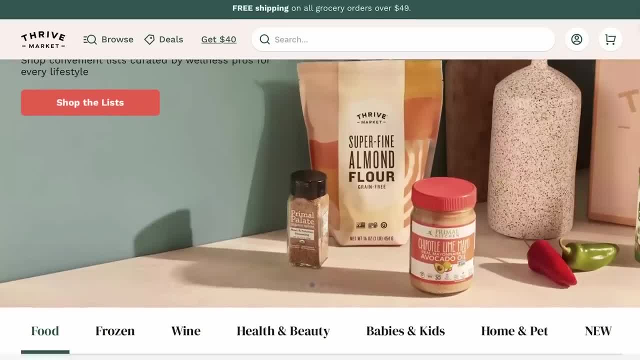 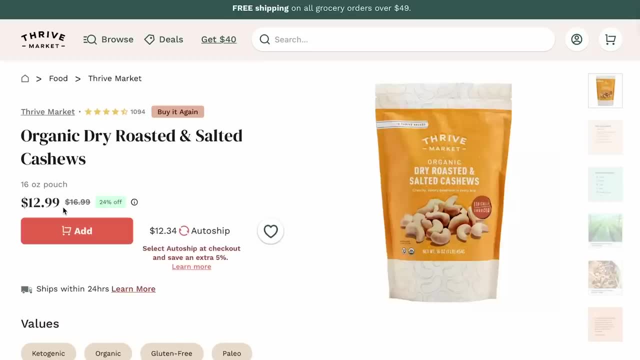 And if you're interested in joining Thrive, you can choose your membership term. I go with a 12-month membership, which comes down to $5 a month, but if you're not sure and you just wanna try Thrive, you can choose a shorter term. 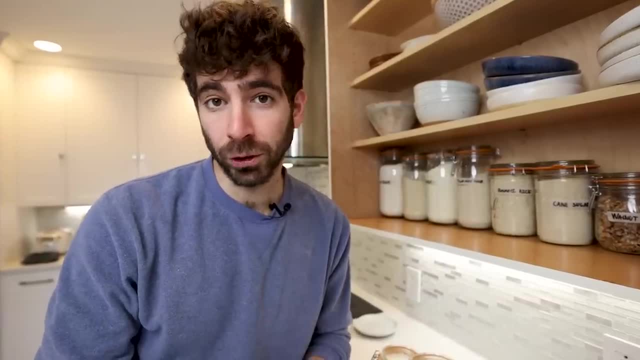 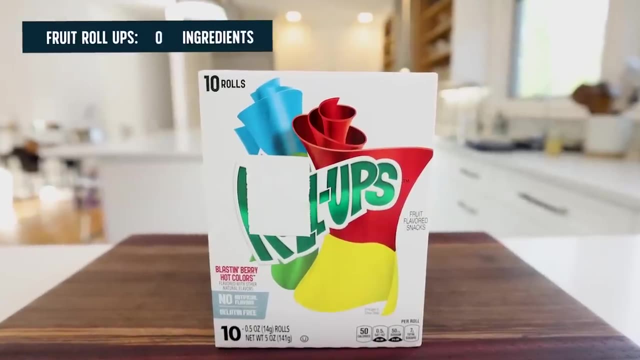 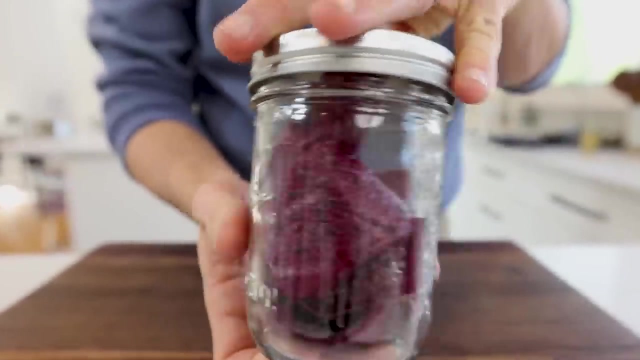 And you can use the link below in my description to get 40% off your first order and a free gift when you join Thrive Market today. Now back to some more snacks. All right, I am making dragon roll fruit roll-ups. 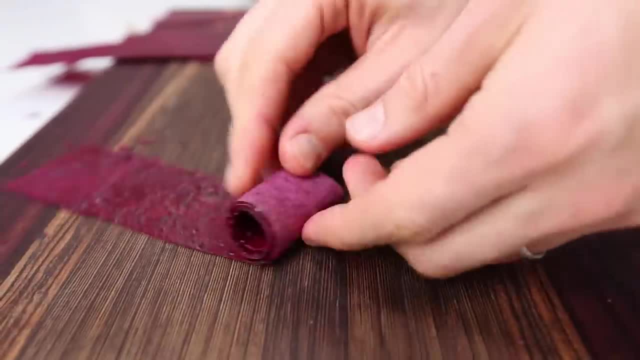 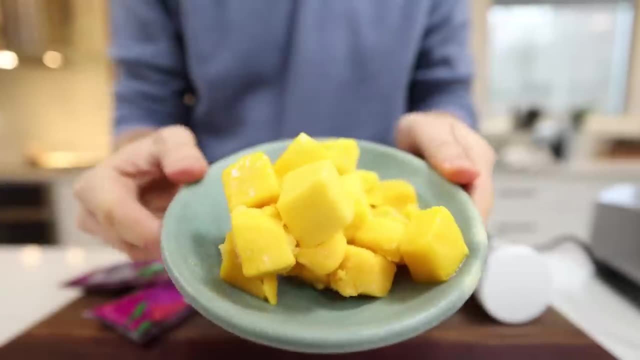 No, that doesn't make sense. I'm making dragon fruit roll-ups And guess what? This is only four ingredients, which is insane. It does come with a longer cooking time, but the actual prep couldn't be easier. You can use any fresh fruit or frozen fruit. 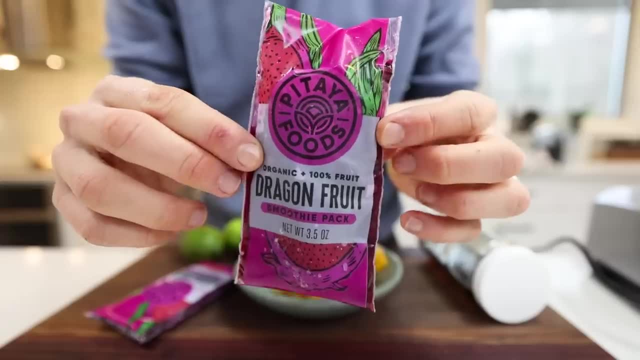 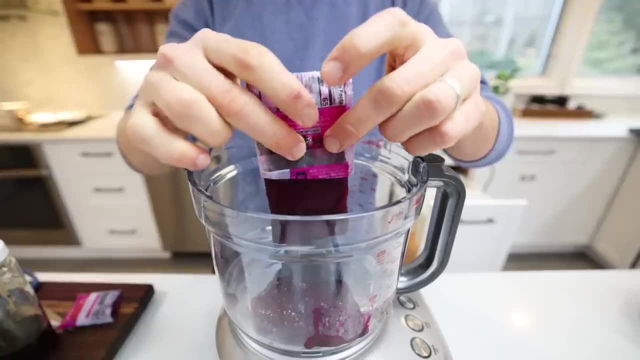 to make a fruit leather, I'm gonna go with frozen fruit And to really ramp it up a notch, I'm gonna use some dragon fruit or pitaya. So I'll dump out two packets of that into a food processor, along with some frozen mango to just bulk it up. 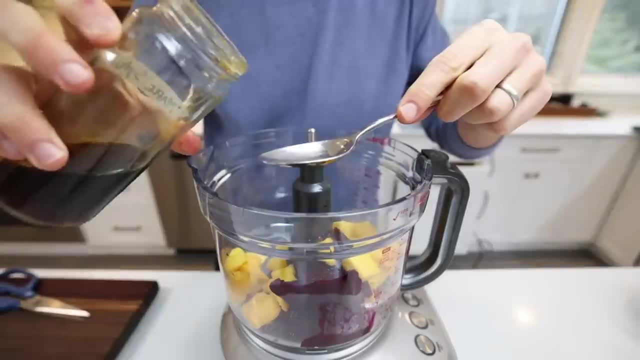 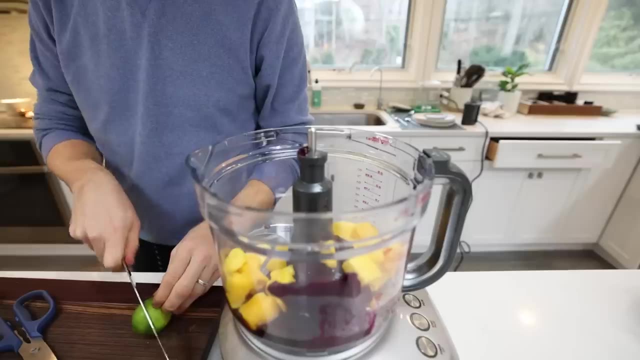 and balance out that tropical flavor. Now I'm gonna hit it with some maple syrup, which is optional, But if you want this to resemble candy, well, a little extra sweetener won't hurt. Finally, I'm gonna squeeze in some lime juice. 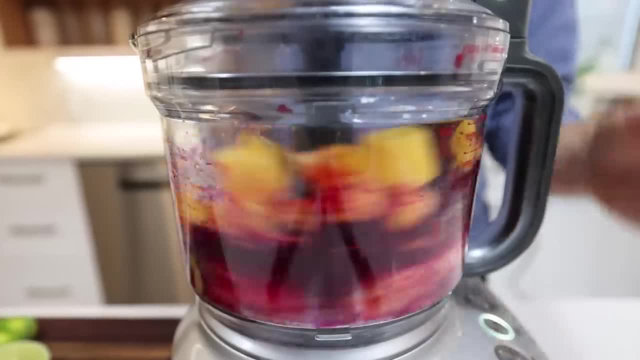 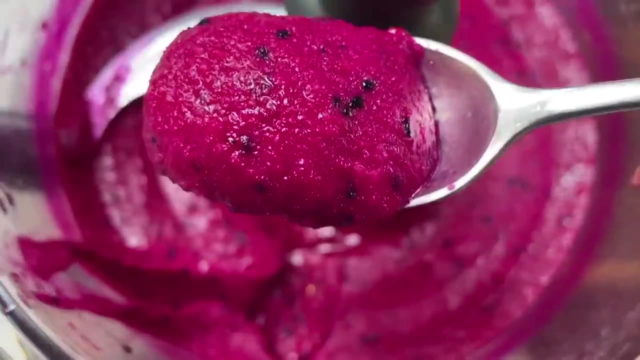 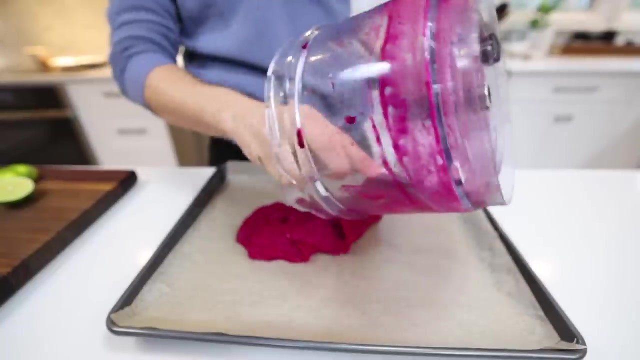 to really just kick up the flavor and give a little bite to these fruit roll-ups. Look at the color on that. That's why I love using dragon fruit. Now, this can be a little tricky to smooth out, but just do your best. 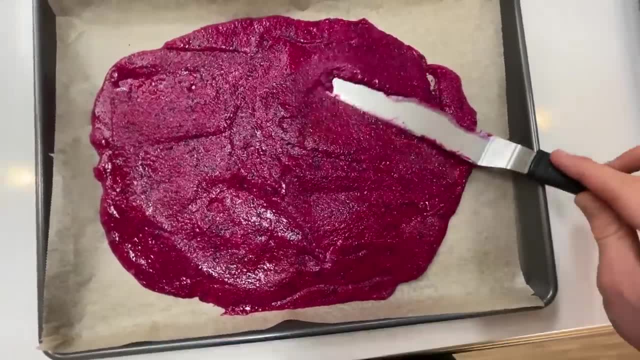 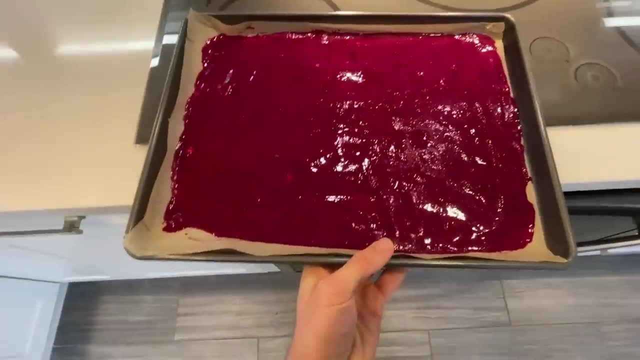 And in the end it will all even out once it sits there for a minute. All right, so we have our even layer of dragon fruit mango puree. Now you can set your oven at a higher temperature if you want this to cook faster. 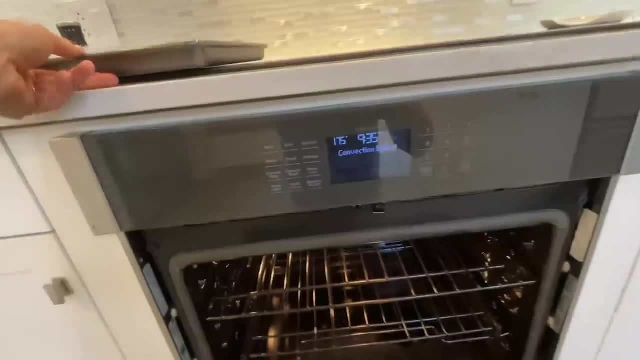 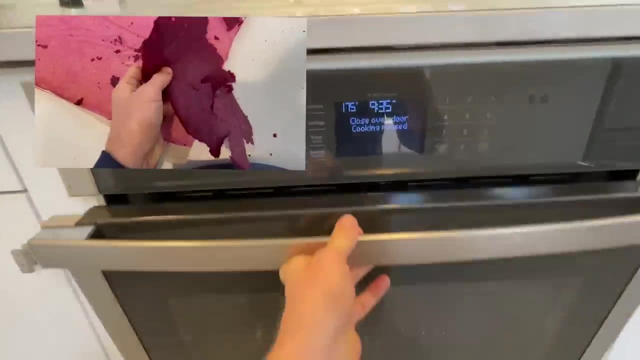 Say 275 Fahrenheit, it will cook in two hours. But at those higher temperatures the sugars will caramelize and you'll get something like this right here. If you choose the low and slow, like 175 Fahrenheit, you're not really cooking at this temperature. 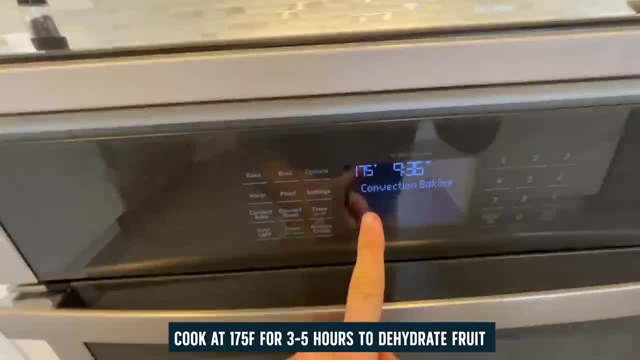 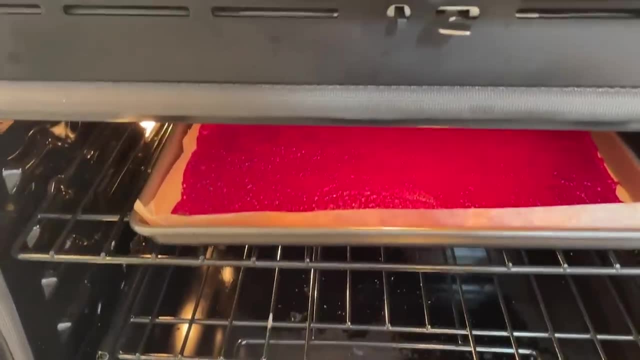 You're more dehydrating So it'll take a little longer, but you'll get a nice chewy fruit roll-up texture. I'll set it for two hours and check back then, All right, so it's been about two hours on this dragon fruit at 175.. 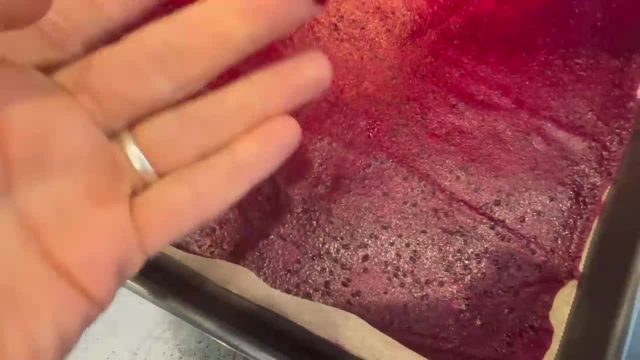 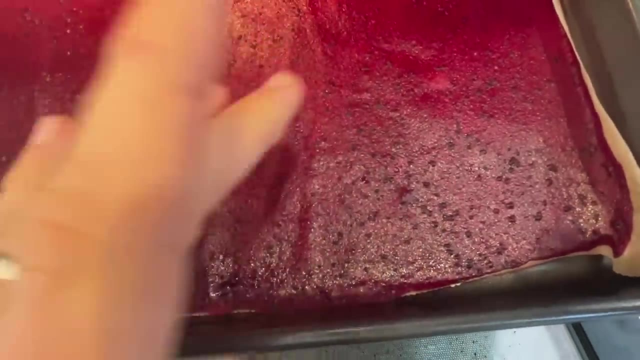 Let's touch this. It's really not that hot, Okay, so, yeah, not totally dry there, But if I touch a corner, yeah, the corners are tacky and pretty much dry. Honestly, another 30 minutes to an hour. 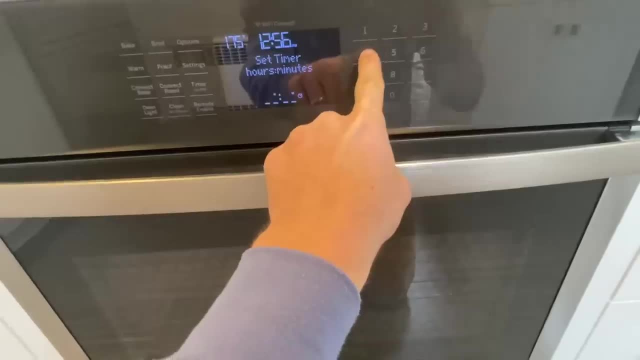 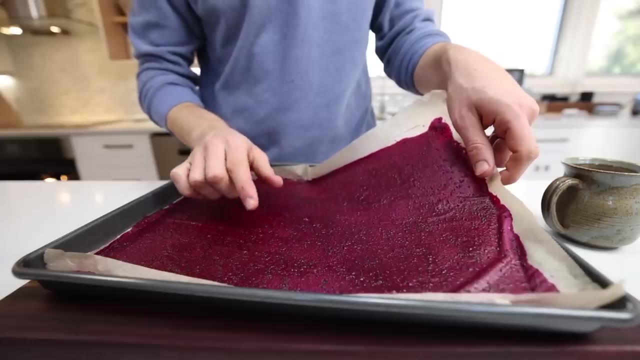 these should be good. Oops timer, We'll set it for 45.. All right, finally we're out of the oven. Maybe a few spots that are still a little moist. We've got a solid, pliable sheet of dragon fruit. 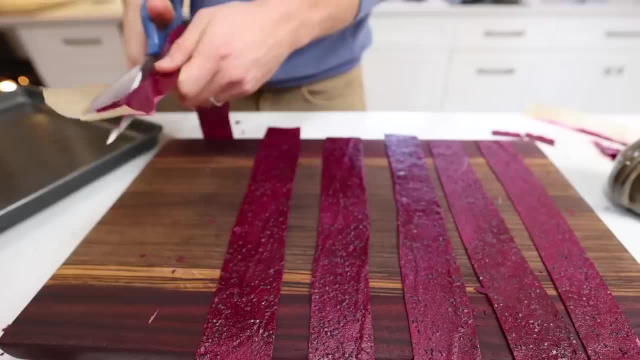 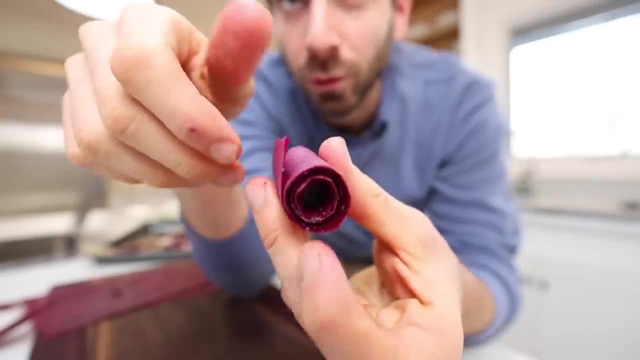 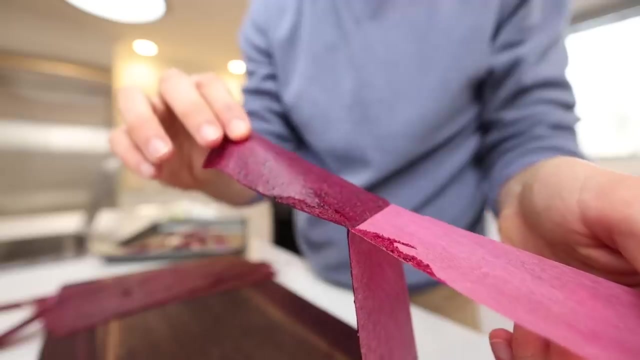 Just gonna cut some strips. All right, now check this action. We've got our dragon fruit, mango fruit roll-up. Give it an unroll Boom, Parchment paper still on the back, A magical unwrapping. Oh, we're losing it. 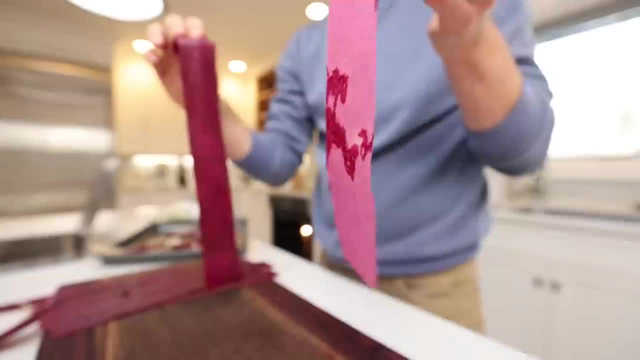 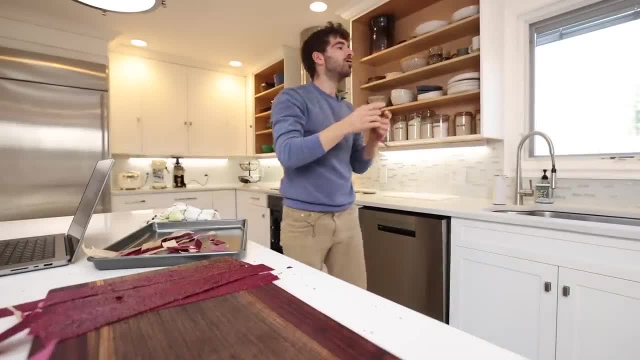 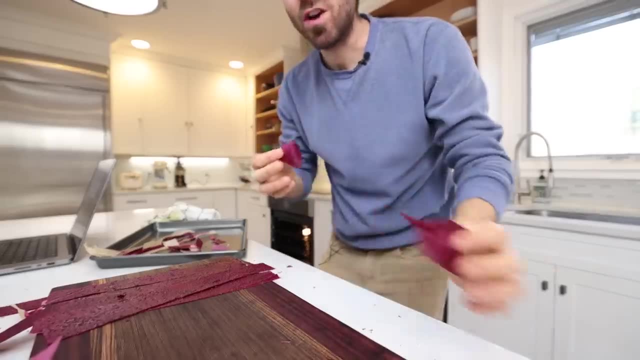 Okay, and the official taste test. Oh my God. First of all, inhaled that fruit roll-up in three seconds. I mean, I haven't had an actual fruit roll-up in maybe 25 years, which is insane to say, But that's incredible. 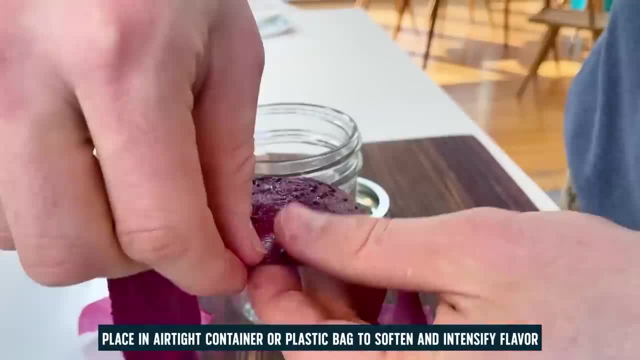 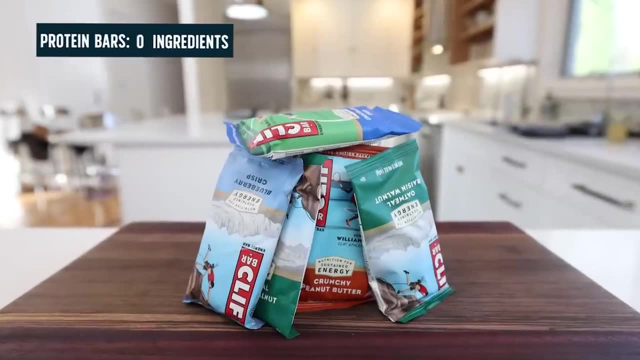 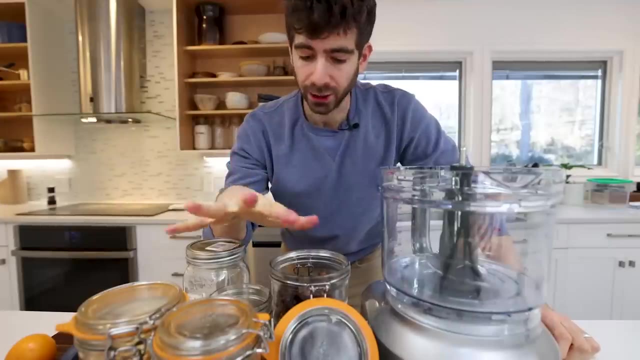 Plenty, sweet enough, just from the natural fruit and a little maple syrup- Very tropical and exotic- from the dragon fruit And just a few ingredients. So these are my go-to because they're very customizable with whatever you have in your pantry And my daughter loves them, which is a huge bonus. 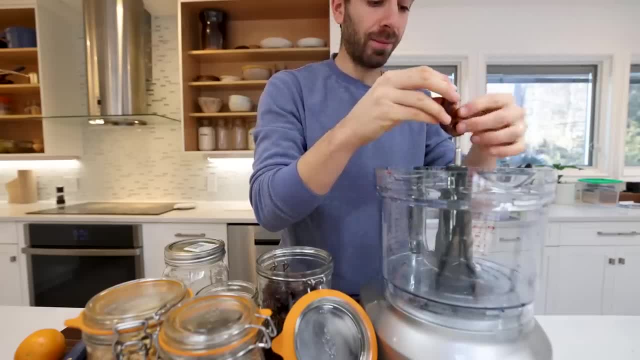 Now I'm just gonna go rough measurements here, which I always do when I make anything in the kitchen, really including these energy balls. But if you want specifics, just click the block. And I'm just gonna go rough measurements here, which I always do when I make anything in the kitchen, really including these energy balls. 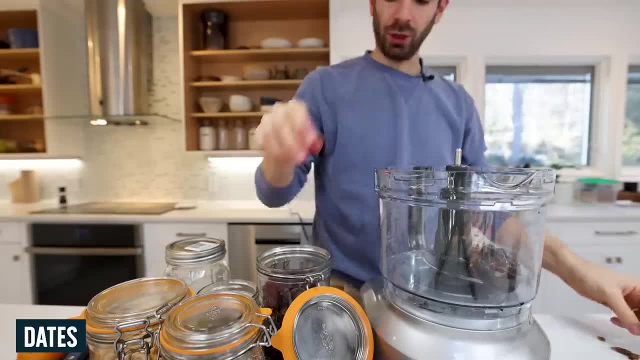 But if you want specifics, just click the block. And I'm just gonna go rough measurements here, which I always do when I make anything in the kitchen, really including these energy balls. So the dates really are your glue and your sweetener. 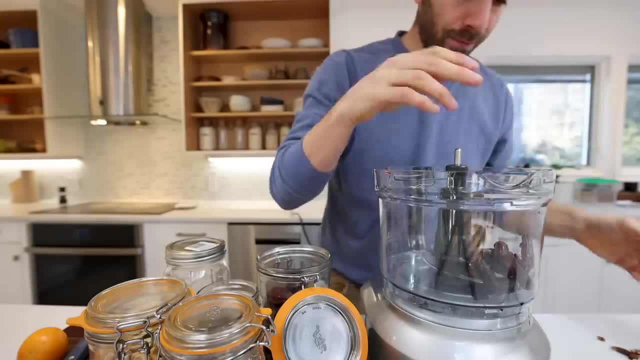 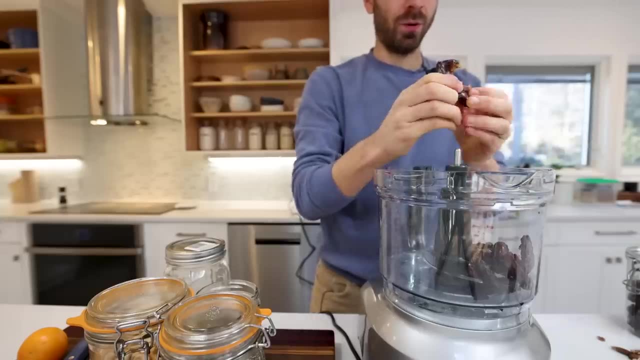 That's one ingredient you can't skip, And I generally start off with about six or seven metajoule dates. They're nice and sticky And nature's caramel. You know what? I wanna go? one more boop. Just make sure you take out your seeds. 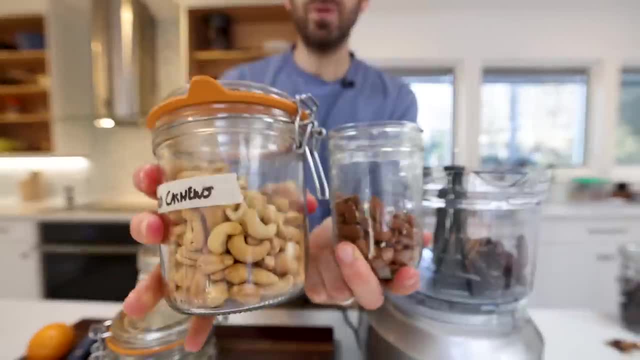 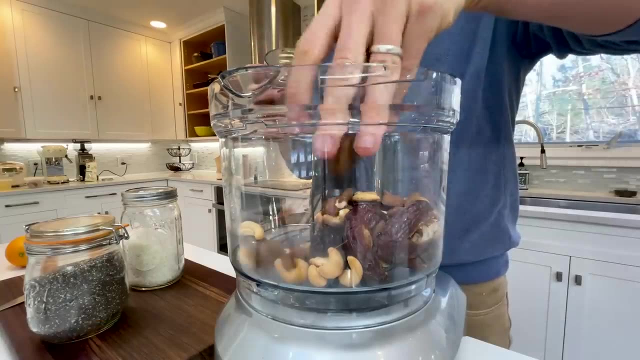 or your food processor's really gonna feel it. Next layer: we've got our nuts. I'm going with almonds and cashews. Got a handful of cashews roasted and a handful of almonds. Got a handful of cashews roasted and a handful of almonds. 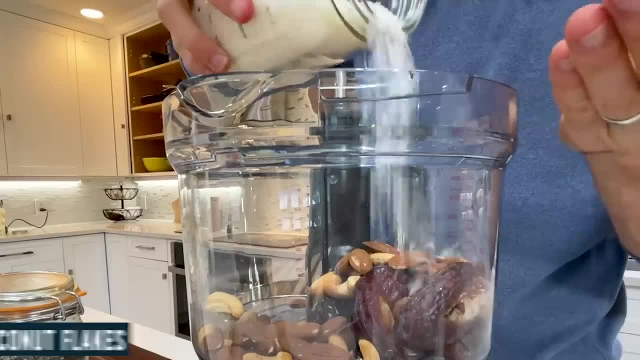 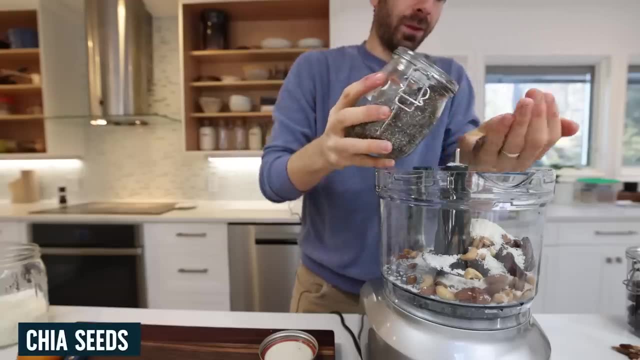 These are actually unroasted raw almonds. Love me. some coconut in there. Same thing. just a handful and a half of those. And then finally some chia seeds- half handful of those. Now we'll process. It's gonna be rough at first. 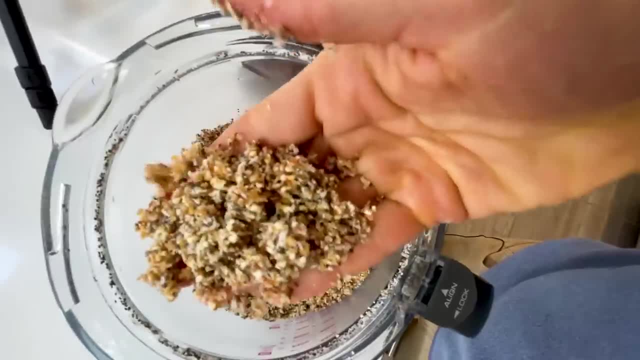 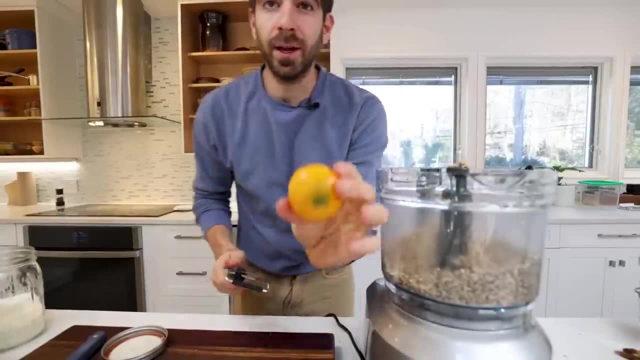 Give it some time. If you take a look in here, beautifully processed, nice and even, but this is crumbly, falls apart too easily. So to bring everything together plus a final touch of flavor, just any orange or clementine. 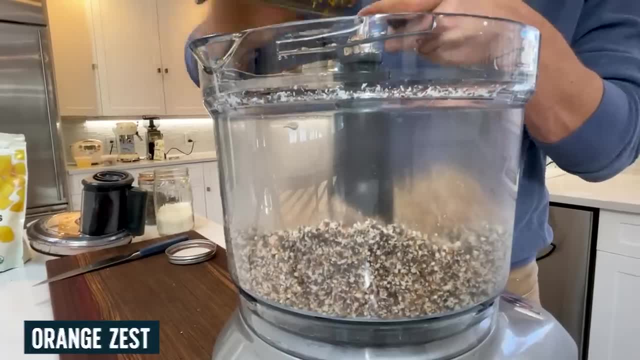 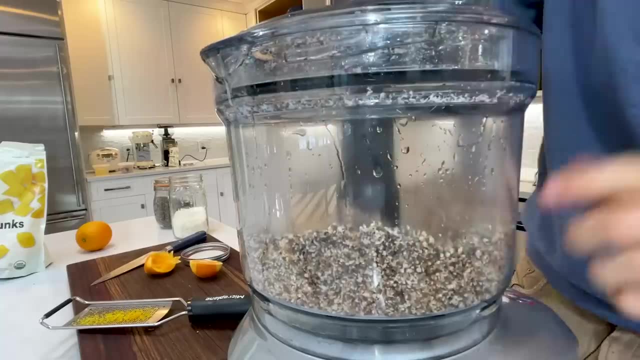 I'll zest first, which really boosts the flavor on these, And then I'll slice, and I'll start off with just half a juice of lemon, Half a juice of orange, And then we'll just give it a few pulses. Now you can see how it's clumping together all on its own. 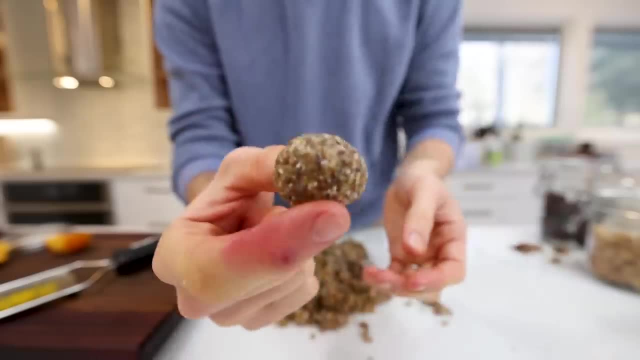 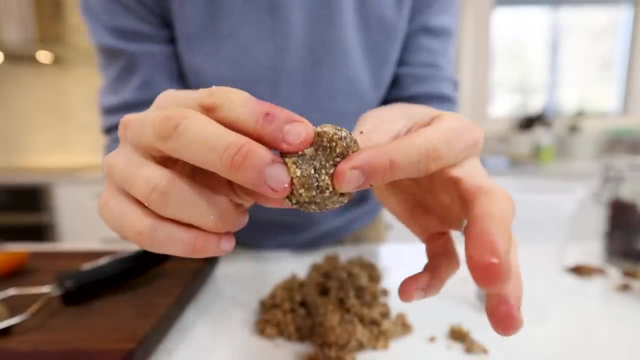 That's what you want Now. some quick manual labor. That's all it takes. Make them whatever size you want, but that is perfect, And I'll actually refrigerate these. You can eat these right now. They're delicious, but they're pretty soft, bit mushy. 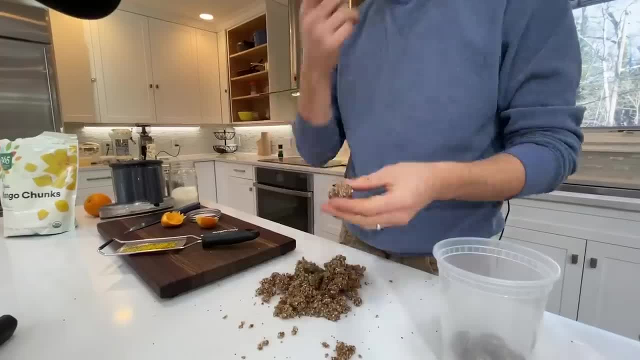 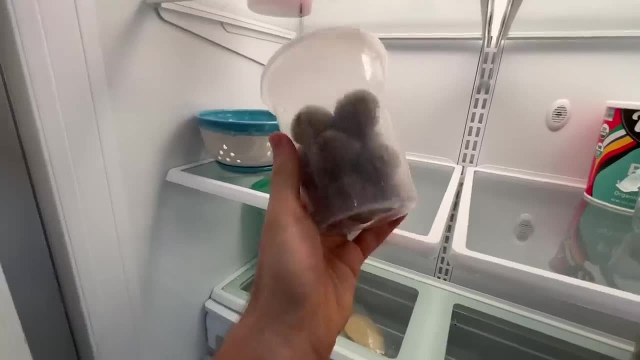 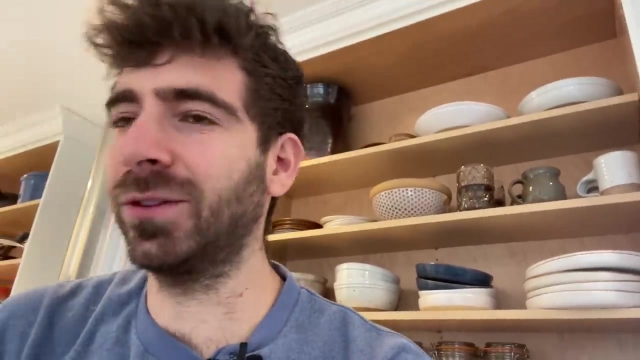 But when you refrigerate them they become the perfect texture. So these will keep in the fridge for a while, but my guess is you'll finish them in a day or two. I find that when I have these energy balls around, it's not so much that they're giving me energy. 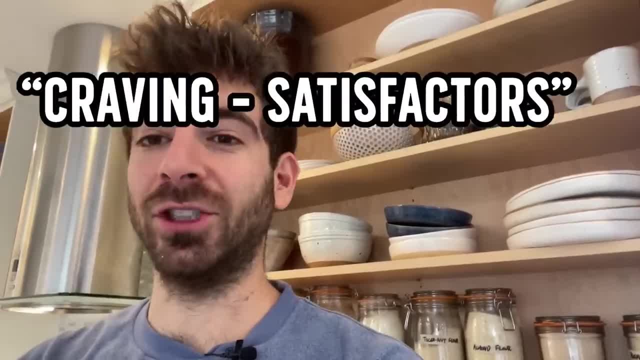 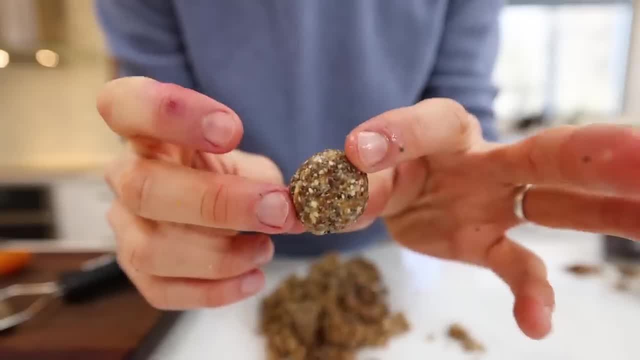 It's kind of a ridiculous term for these. They're more like craving satisfactors. They're sweet, they're a little salty, they're filling, So I just snack better when I prepared those at the beginning of the week: Energy ball. 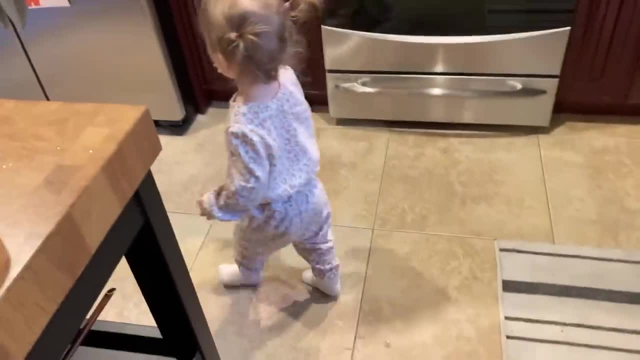 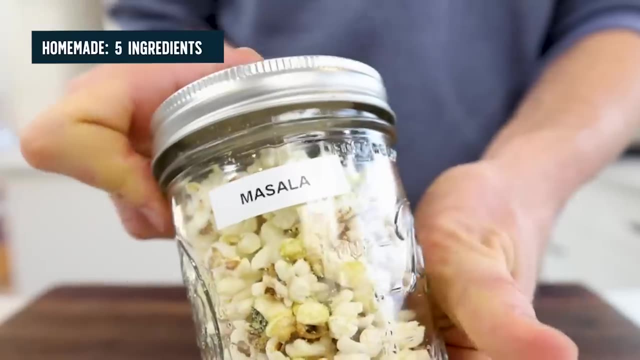 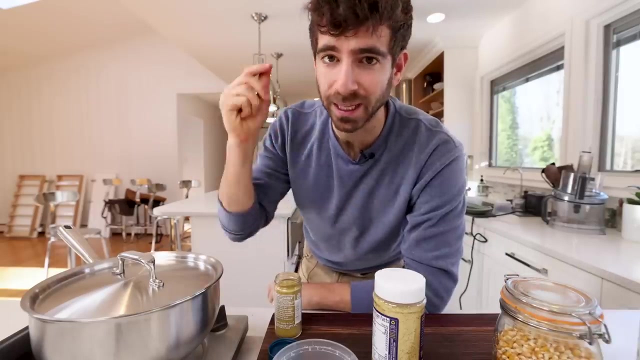 Energy ball. And finally, well, every Pro-Am cook should definitely be making popcorn from scratch. But, more importantly, you need that one spice mix that makes popcorn extra consumable, And this cheesy spice. at this point, I don't make popcorn without it. 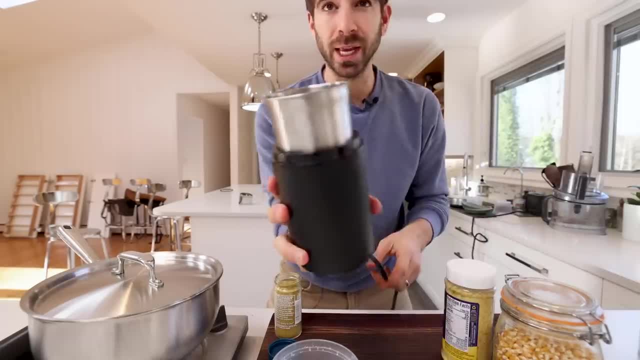 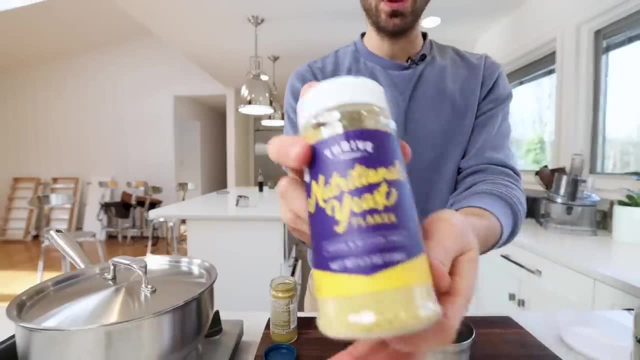 just because it's so damn addictive and really simple. So I'm using a spice grinder here, but if you use all powdered spice, you can just mix them together, Okay. so the star of the show- nutritional yeast. That's gonna give it its cheesy flavor. 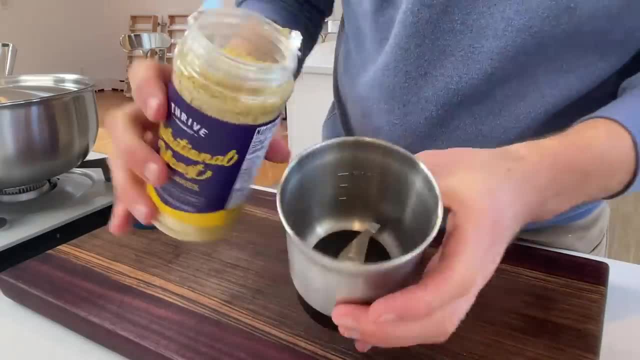 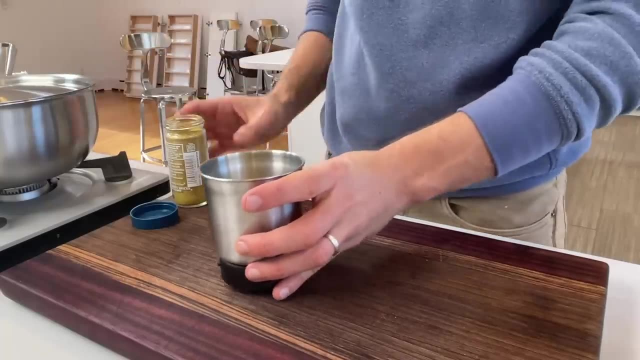 and just a lot of sort of natural umami in here. Now this is gonna make up about 75% of the spice mix, And really the additional stuff is just extra flavor. Sesame seeds might seem a little crazy When blended up. I love the sesame flavor in there. 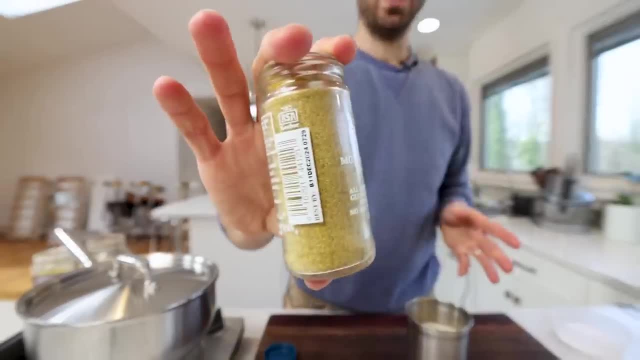 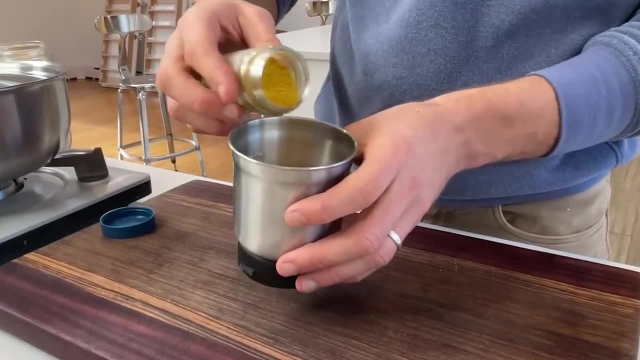 I stumbled across that one day just kind of randomly, and it worked great. Now here is a curry powder, A little bit of that. You can use any ground spice, though, if you want some garlic flavor, or onion powder. And then, finally, it needs a good bit of salt. 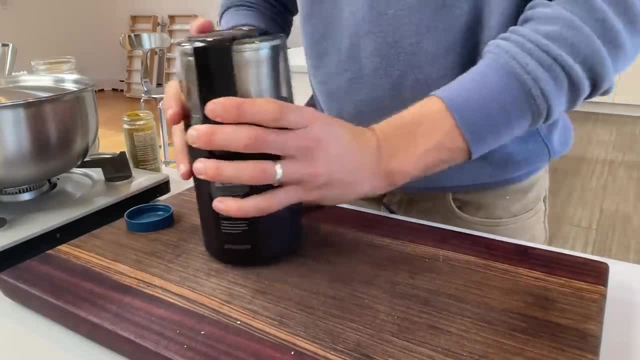 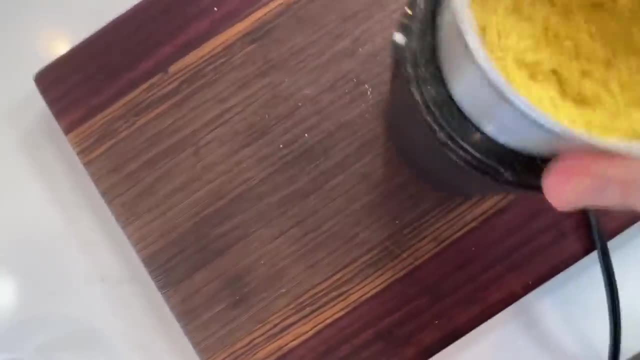 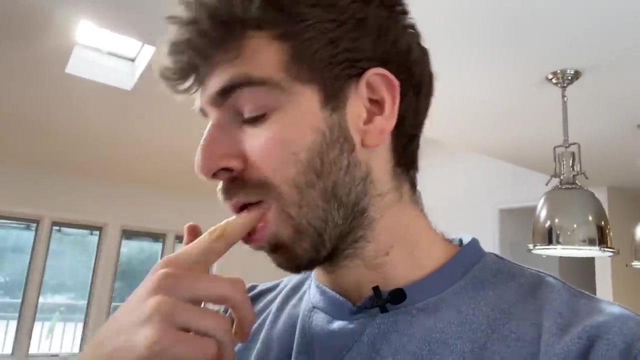 It is a spice mix. after all, Sesame seeds still need some work. Now, one thing about using a spice grinder is you can get it super fine, so it creates a nice powdery coating on your popcorn. You want those Cheeto fingers? 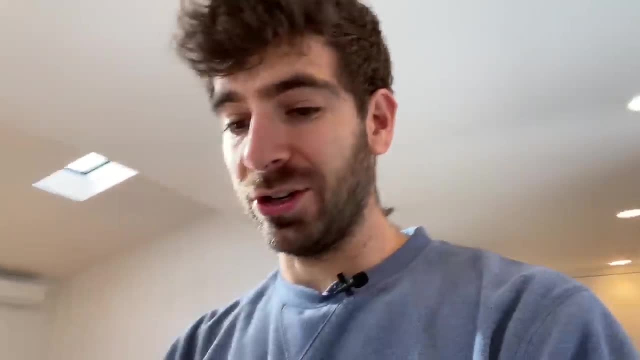 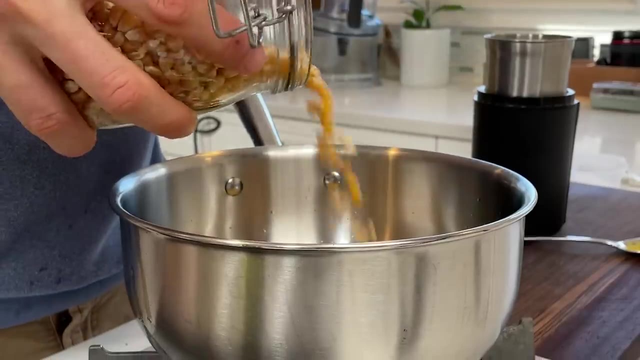 It should pack a nice punch. That's cheesy, that's salty, that's goodness. Let's make some popcorn. Medium heat, little bit of oil, Popcorn- Really, you just wanna coat the bottom of your saucepan. One even layer.